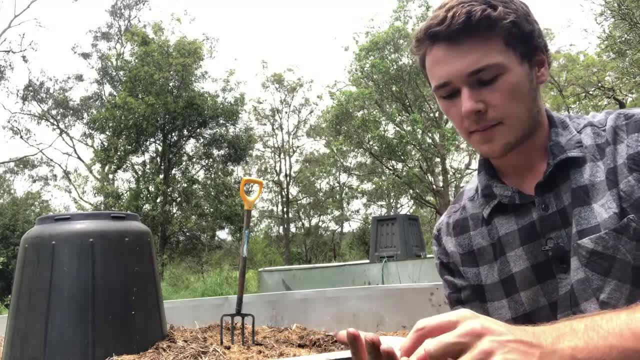 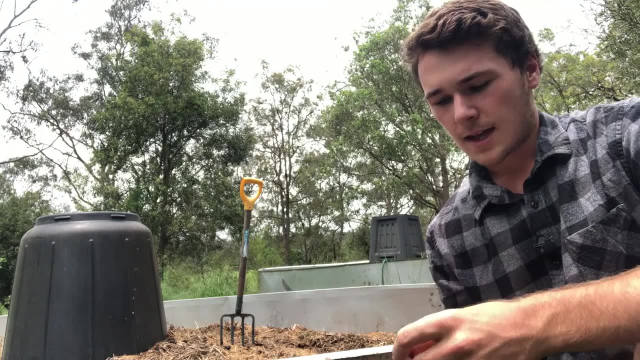 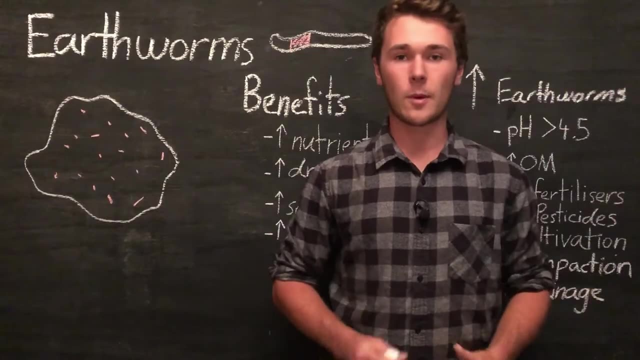 In this video we'll be looking at the benefits of these earthworms and how essentially they function within our soil and how we can improve their population size. My name is Till Simmons, from AgriSoil, and this is Agriculture Explained. Earthworms are a great way to build healthy soil. 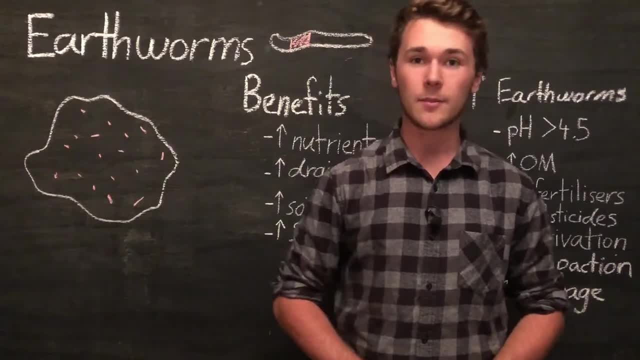 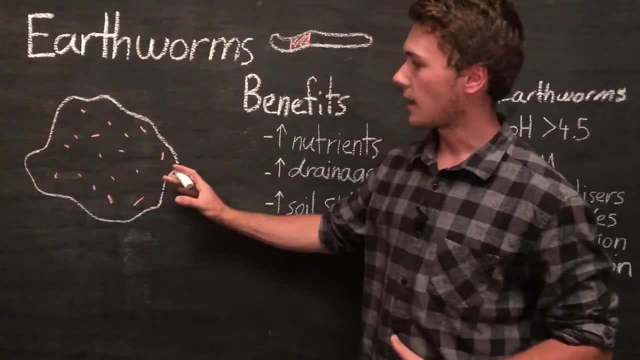 If you see earthworms in your veggie garden or in the soil on your farm, it will indicate that you have healthy, functioning soil. Essentially, what earthworms do is they come across, say, a bit of soil with bits of organic matter in them, and they will pretty much move through the soil and eat. 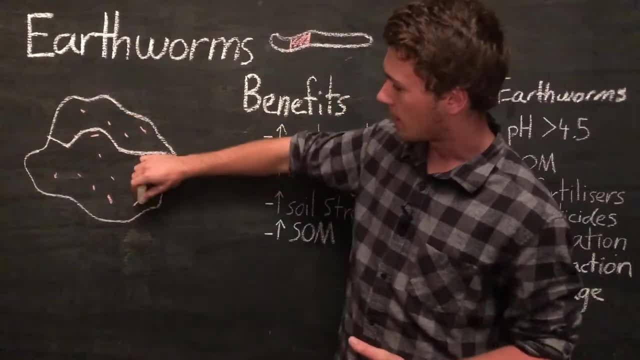 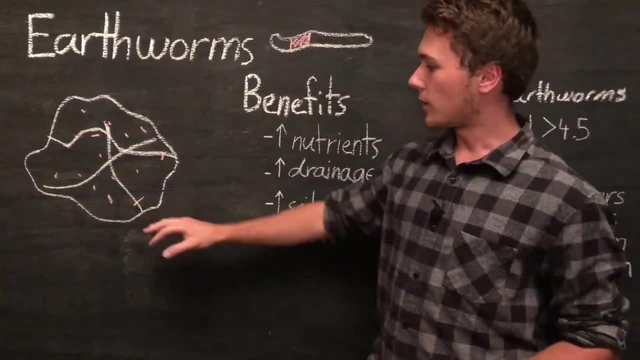 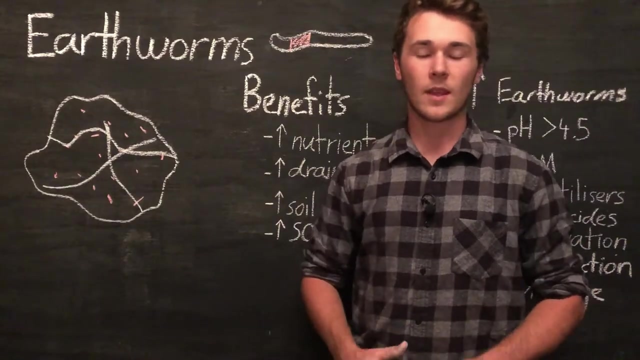 this organic matter. Now, over time, they'll do this a lot and make tunnels all through the soil. While doing this, they're eating all that organic matter. Now, as they eat this organic matter, they digest it and they concentrate the nutrients and then they essentially poop it out as humus. 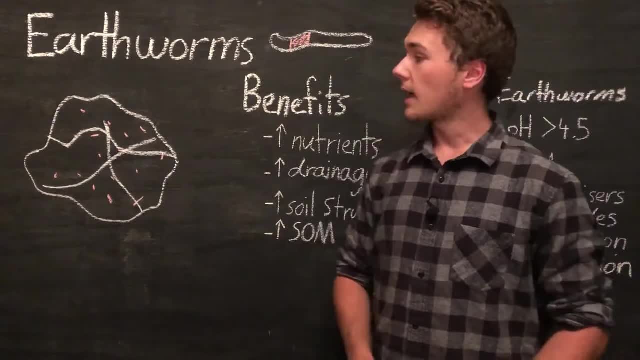 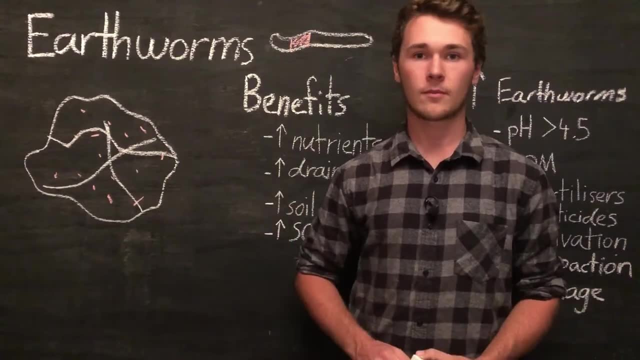 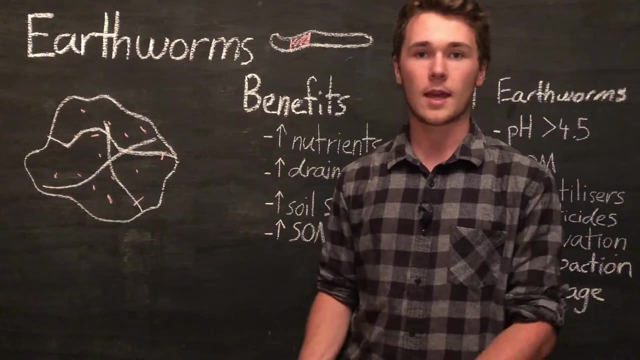 Now, humus is a really nutrient-dense substance, And a lot of the compounds in humus is readily available for plants to absorb. So, as a result, this humus, or also called worm castings, is a great way of giving nutrients to our 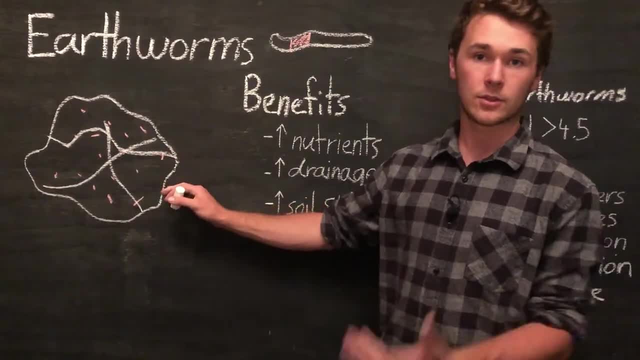 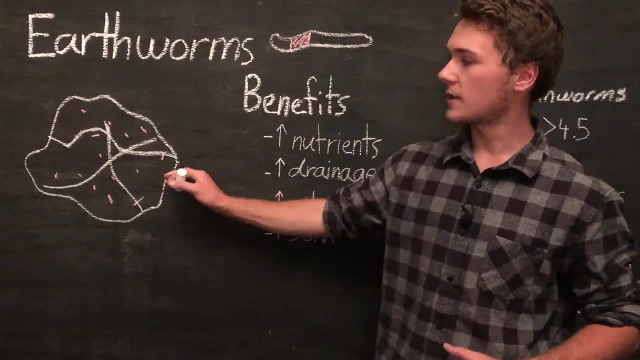 plants by recycling the organic matter already in our soil. So we can see that with the benefits of earthworms they increase the nutrients. So, as we said over here, it just takes organic matter and the nutrients already in that and it converts it into a more. 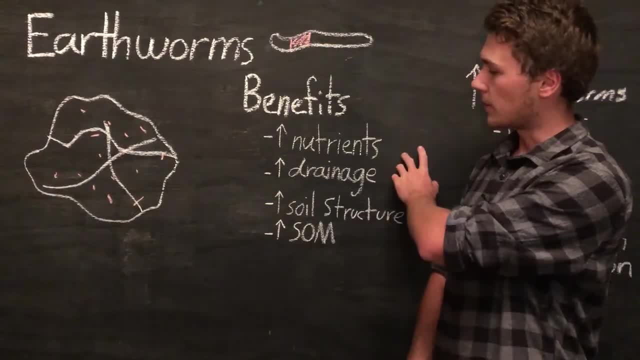 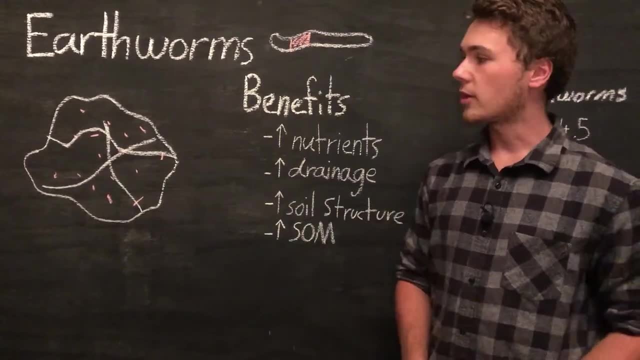 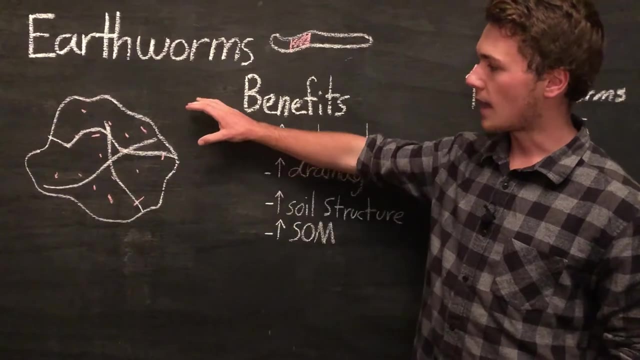 readily available nutrient, So it increases nutrients availability. As the worms move through the soil, it creates these tunnels. Now these tunnels increase the drainage of our soil, So it reduces water logging. and it also increases the gas exchange, So gas is allowed to move through these tunnels and that can help to aerate some of the soil. 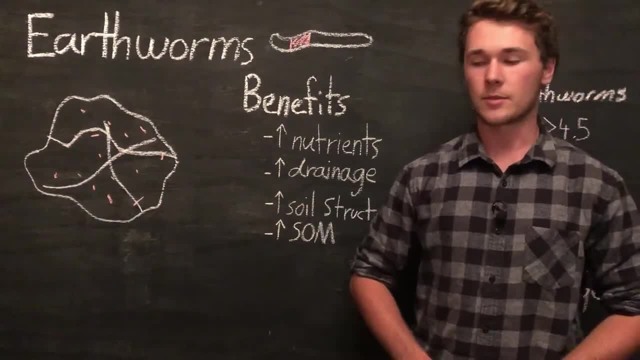 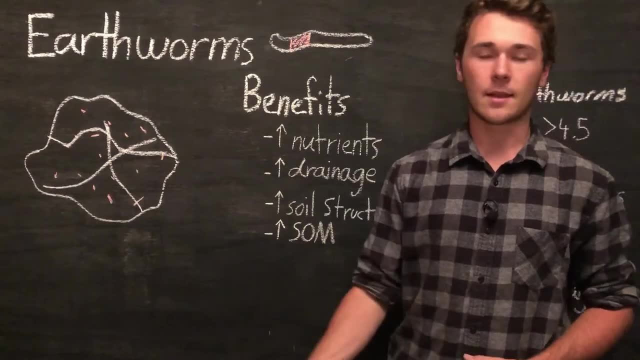 Next is that the castings, or humus release that will bond to soil particles and allow them to come together, So that will increase the nutrient availability. Worms in turn will increase the soil structure. That has a number of benefits associated with that. 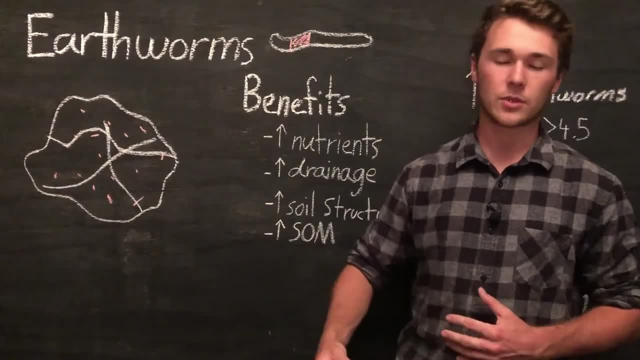 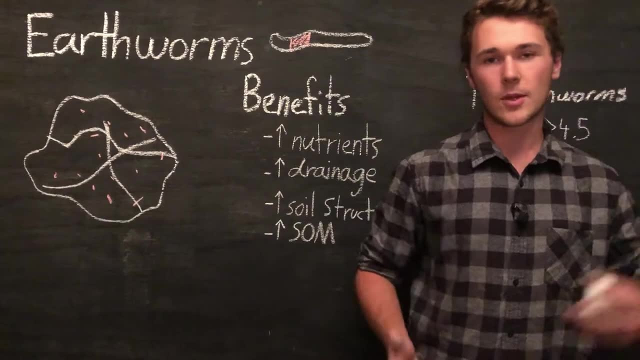 such as water holding capacity, And the humus itself will also have a high channel exchange capacity, So it will help to exchange nutrients to the plant. And lastly, with this is that we're going to increase our soils organic matter and, as we know, with the soil organic matter video. 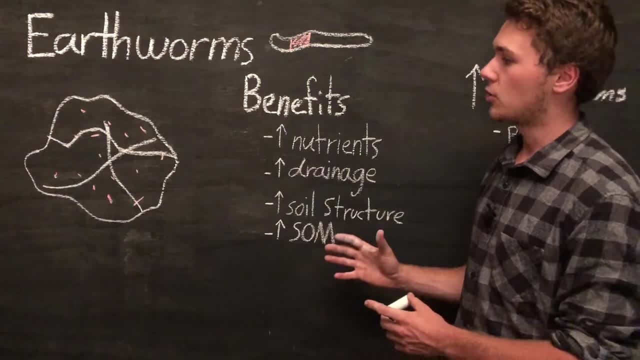 we have a heap of benefits with that. So earthworms contribute so much benefit to our soil And without any extra work to such. Without any work to such. So earthworms contribute so much benefit to our soil And without any extra work to such. 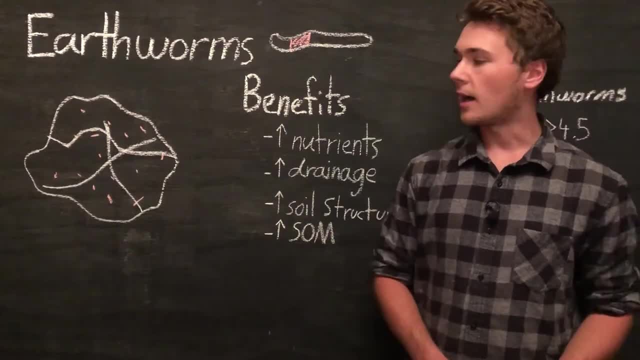 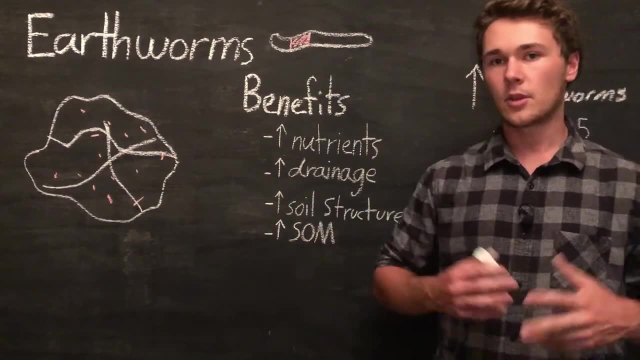 And without any extra work for a And without any extra work to such, because with that extra work, say on our half, We're just going to make sure that we allow for a healthy environment and they will pretty much contribute all these really beneficial aspects to our soil. Now, 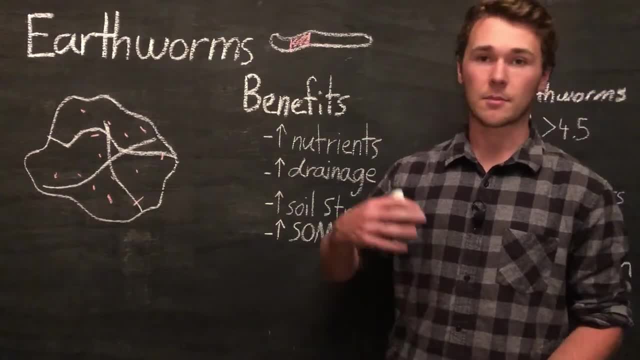 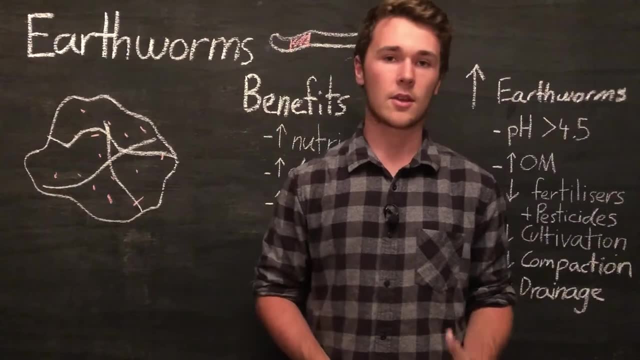 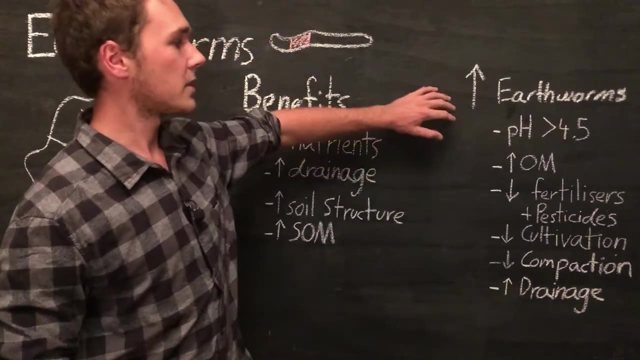 if you don't have many earthworms in your soil, it may be due to some practices or cultural practices that you're using on your farm or veggie garden. Now some of these deter earthworms from living in soil just because they don't like it. So what we can do to increase earthworms? 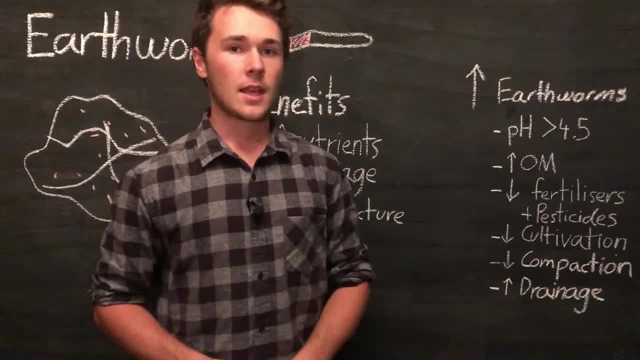 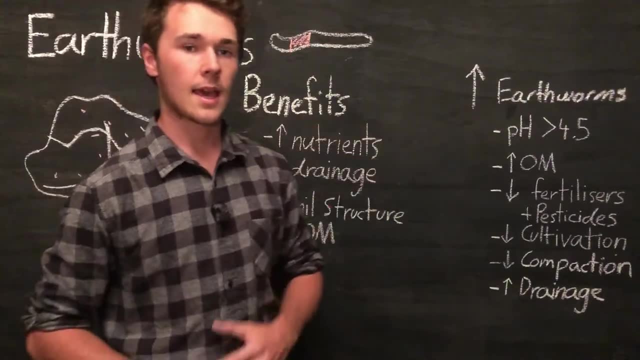 is make sure we have a pH above four and a half. Anything below that's too acidic for them and they're not going to like it. So to do this we just test our soil and then make corrections. So you can either add lime to raise the pH or sometimes a low pH can. 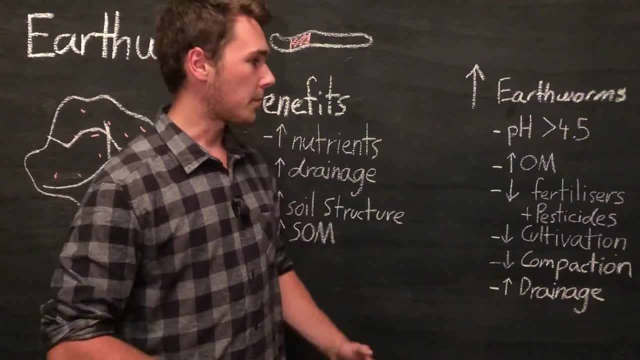 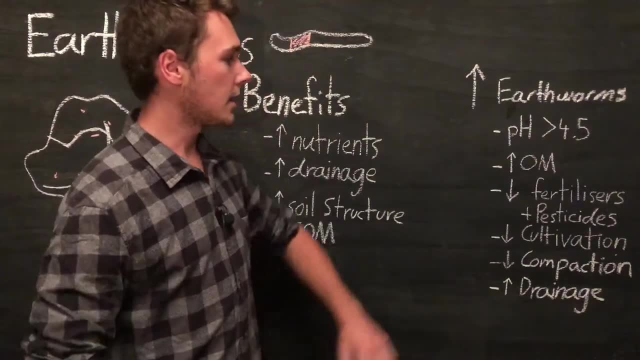 be the result of too much chemical fertiliser applications. So a long term solution is we can reduce our inorganic fertiliser application. Now the earthworms need something to eat, so we can do that. by increasing the oil, We can increase the organic matter. This will promote them to an area because there's feed. 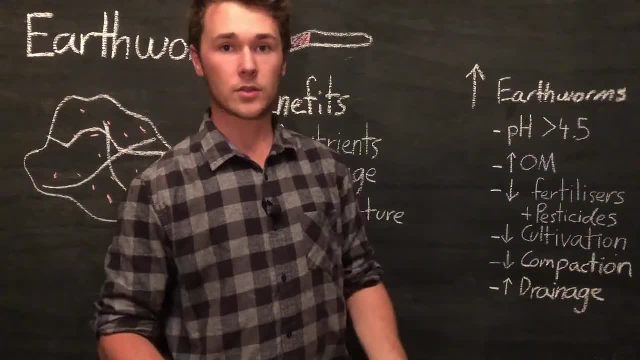 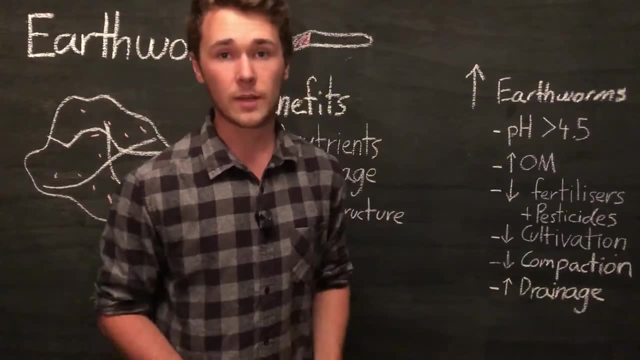 there so they're going to want to be there. We can increase the organic matter within our soil by either planting in a green manure crop- So you just plant a bunch of really leafy plants, pretty much So like oats or sorghum, and then planting that all back- Or 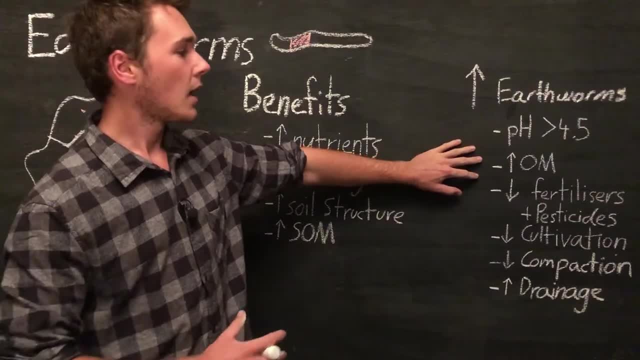 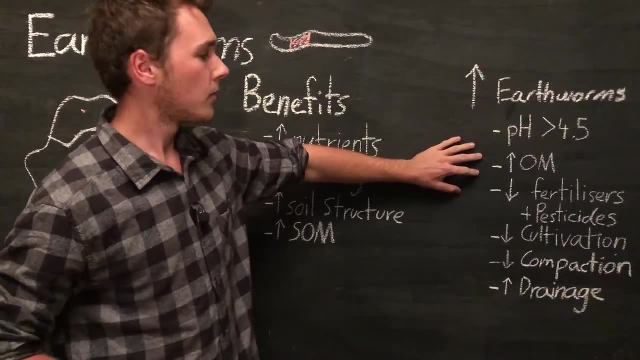 just allowing you don't have to plant it back, but you could also graze that with some livestock and then the manure it will increase the organic matter. We want to decrease fertilisers. So, as I said, with the increase in pH from inorganic fertilisers. 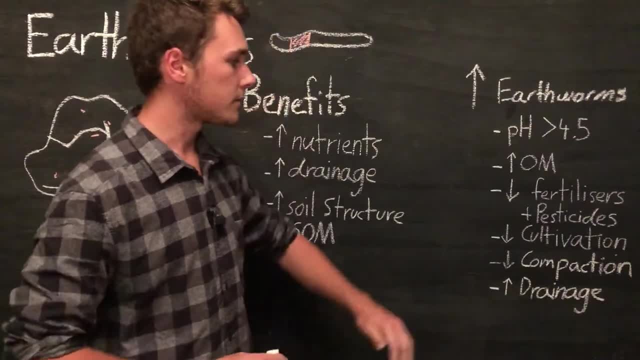 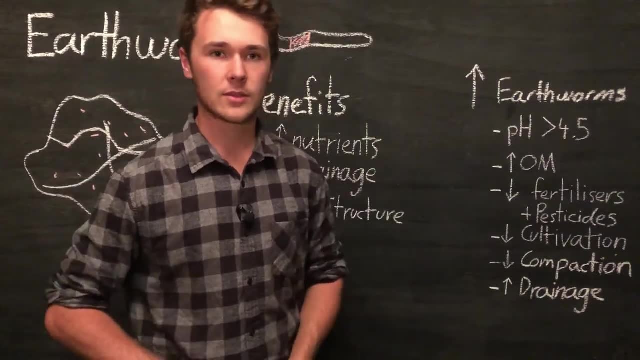 So reducing fertiliser, and definitely the more harsh fertilisers, will promote earthworm population activity, And that's just because a lot of earthworms are really sensitive to their environments. Any harsh chemicals will deter them from living there, As well as pesticides. Pesticides can really harm our earthworms and anything that will harm the earthworms. they don't want to live in that area. So we want to reduce that. Next, we want to reduce cultivation. Now. cultivation disturbs the soil and earthworms don't really. 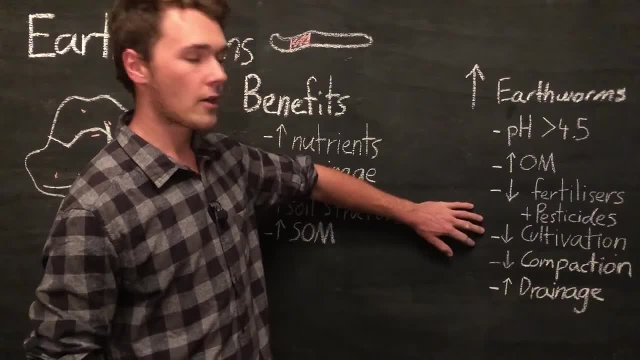 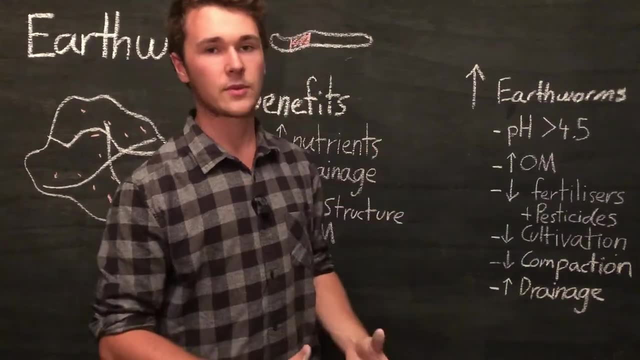 like disturbing the soil too much, So they're not going to want to be in areas that are frequently cultivated. Next, we're going to want to reduce compaction. Now, earthworms find it hard to move through compacted soil, So again, they're not going to want to be there. 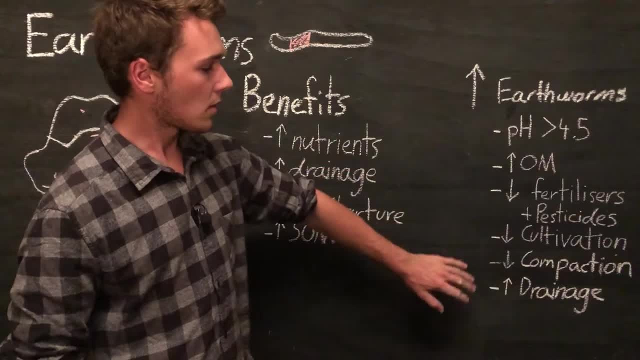 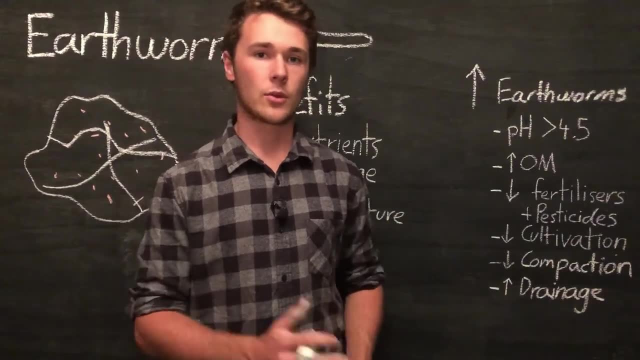 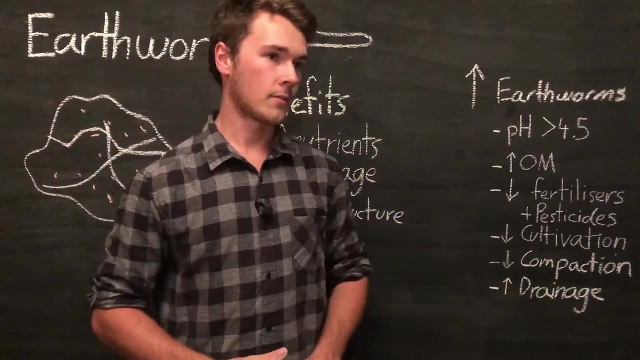 if they can't move through and access their food source. So we can reduce compaction. There's a number of different ways We can reduce compaction and it does depend on what type of enterprise you're running. But moving to a no-till or reduced till, where we're going over the soil less immense time. with our tractors and what not. That will reduce compaction from that. There's a couple of other ways we can reduce compaction naturally with using perennial plants That will permeate deep roots into the soil profile and break up that compaction. Otherwise, if you have, 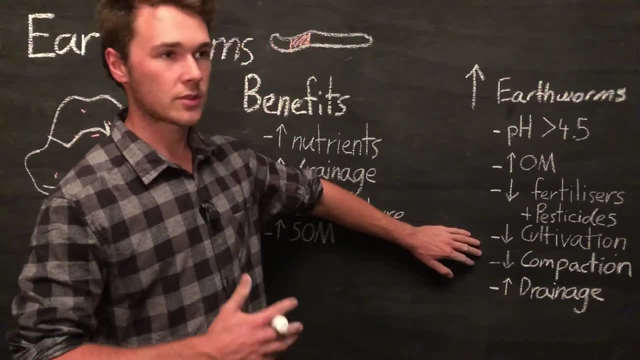 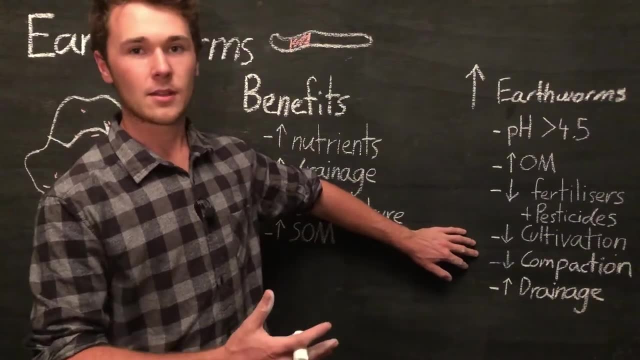 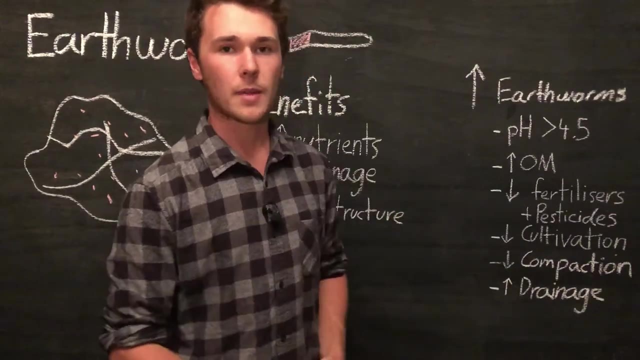 really bad compaction. what you can do is just go through and it is a tilling method, but you get a ripper and they pretty much just rip up the compaction. But the most important thing with that is that once you rip it up you want to make sure you maintain no compaction. 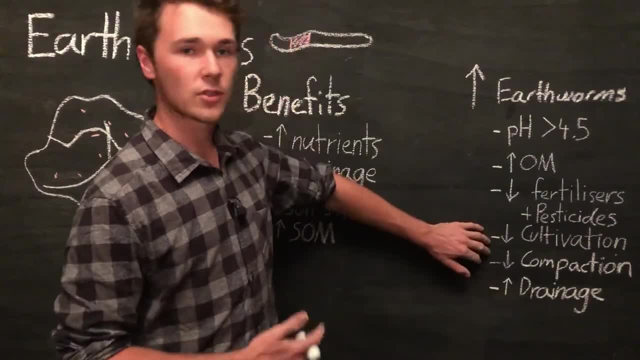 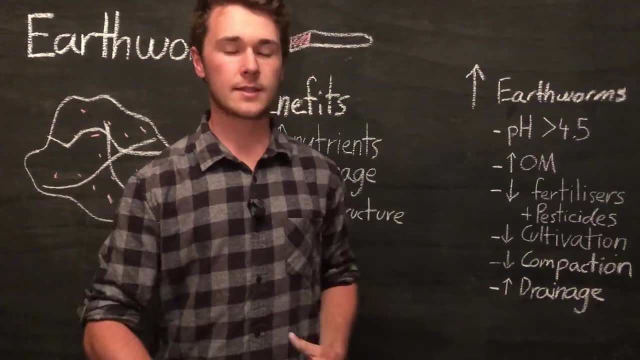 So then you implement different strategies to make sure that you don't reintroduce compaction into your soil. And, lastly, we want to increase drainage because worms don't like super waterlogged environments. Now, it is a bit of a self-fulfilling question. So we're going to increase drainage because worms don't like super waterlogged environments. Now it is a bit of a self-fulfilling question. So we're going to increase drainage because worms don't like super waterlogged environments. So we're going to increase drainage because worms don't like super waterlogged environments. 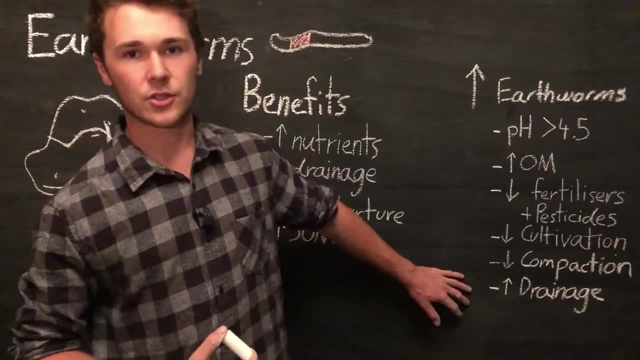 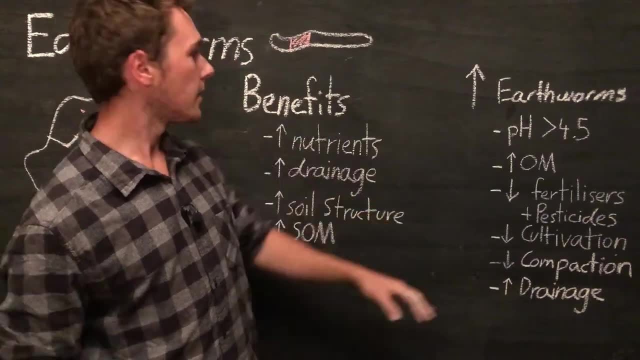 if we increase drainage of, we're going to promote worms to increase drainage, which will increase drainage, and so we get more worms. so it's a positive feedback loop. the better you improve your soil, the more worms you'll pretty much attract to your soil. 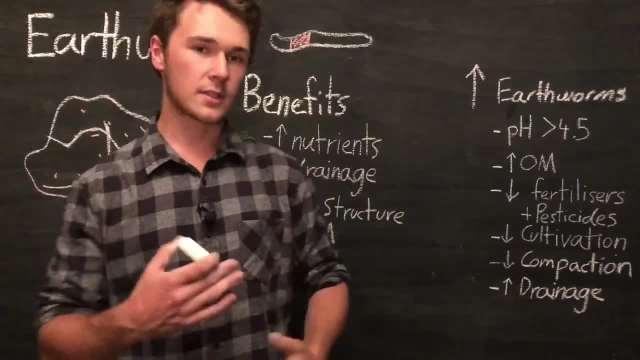 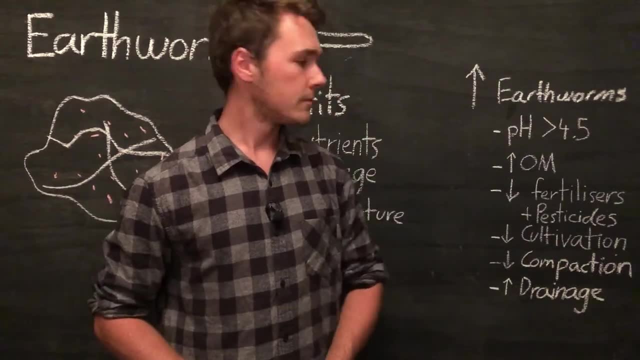 which will improve your soil, which will attract more worms. So once you start getting the more moving of this, you'll say that there's a rapid increase in soil fertility. Now, another point I didn't write off here is that earthworm Od mów assigned, is it's. 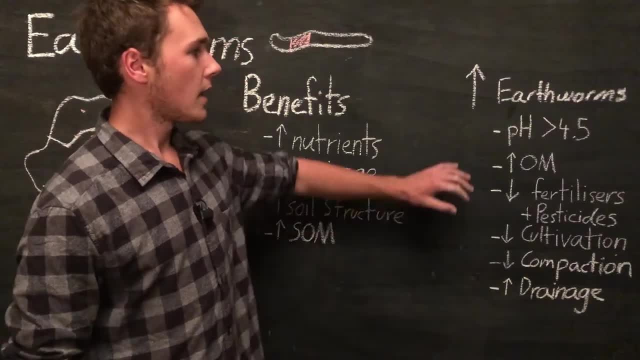 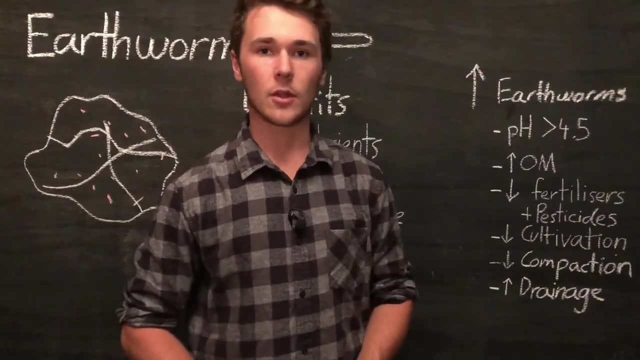 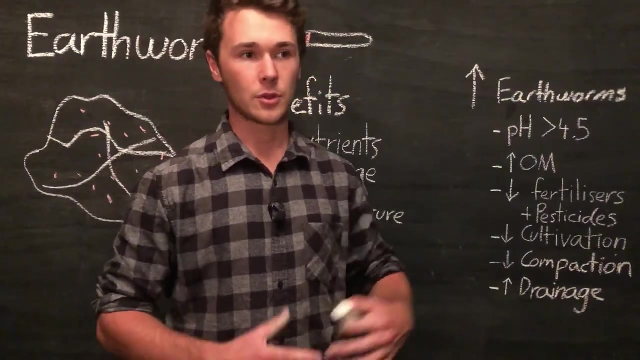 moisture above 20%. so making sure that you have a fair bit of water moisture in your soil to allow earthworms to pretty much be in that environment that they really like. and this is also because earthworms can dry out really easily. so making sure that we have nice moist soil will ensure that they don't dry out now.